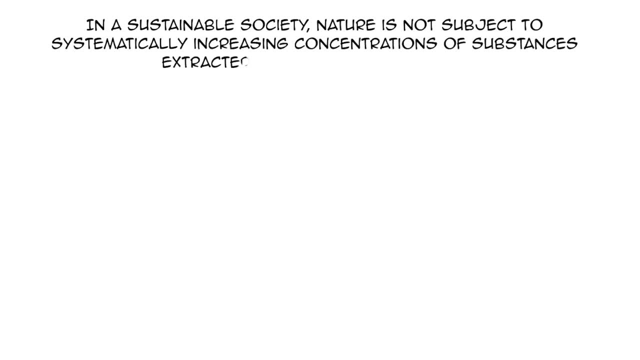 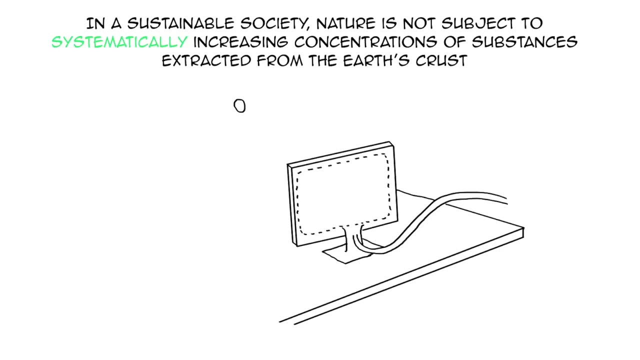 increasing concentrations of substances extracted from the Earth's crust. One important word here is: systematically. Think about it as your email box Say that you get on average 15 emails per day and you have capacity to deal with about 20.. All is well, But one day a colleague of yours takes 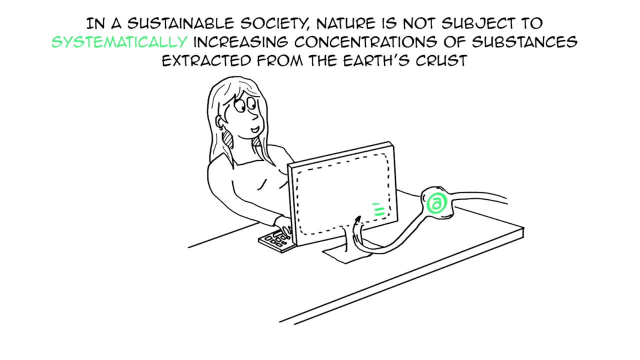 a leave of absence and you get his emails- 15 more emails every day, for a total of 30.. Your capacity is still 20 emails per day. So every day you pile up 10 more unread emails and they systematically accumulate. So this first principle doesn't mean that we cannot use oil. 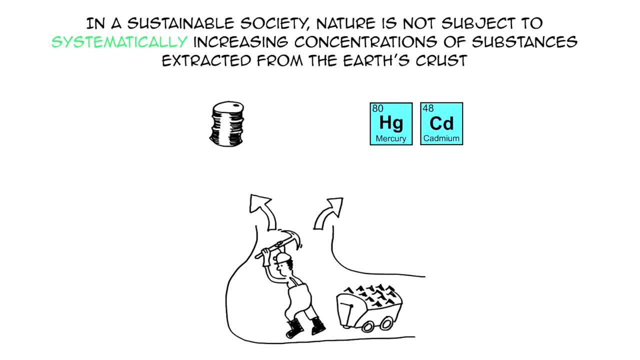 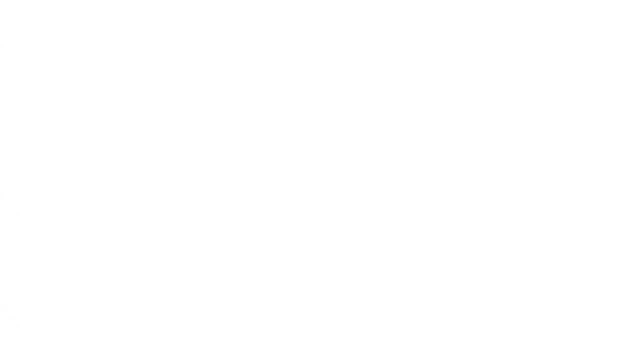 heavy metals or other substances from the Earth's crust. It means that to be truly sustainable, we cannot extract them and build our society in such a way that they systematically accumulate in nature over time, like your emails. The second principle states: in a sustainable society, nature is not subject to. 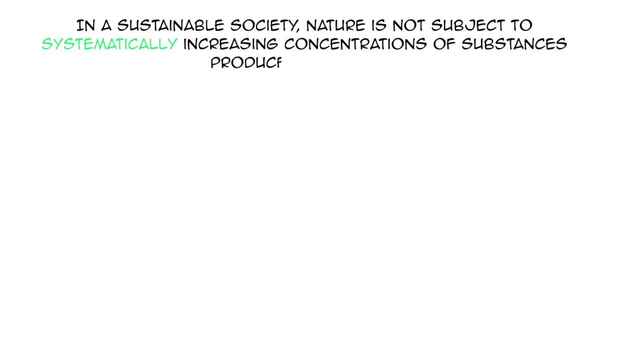 systematically increasing concentrations of substances produced by society. The word substances here refers to chemicals and compounds that nature has either never seen before, like chlorofluorocarbons, also known as CFC, or has only seen in a relatively small amounts. This doesn't mean that we cannot produce substances in society. It 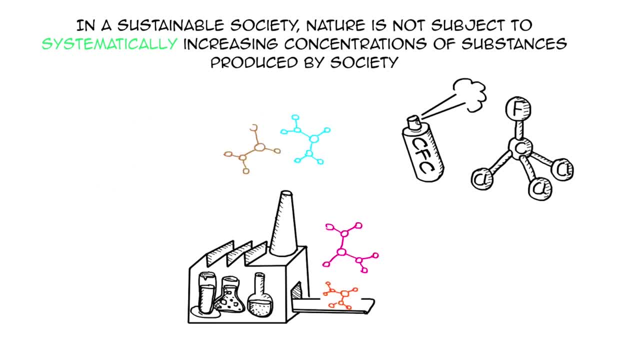 means that, to be truly sustainable, we have to use substances that nature can easily break down, so they won't systematically accumulate in natural systems over time, And that we only release them into nature at a rate at which nature can cope with them, like the emails in your mailbox. 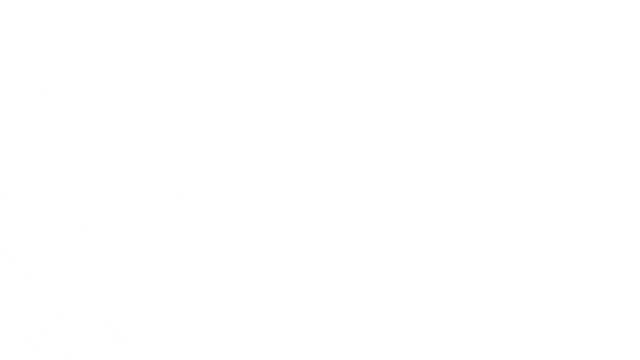 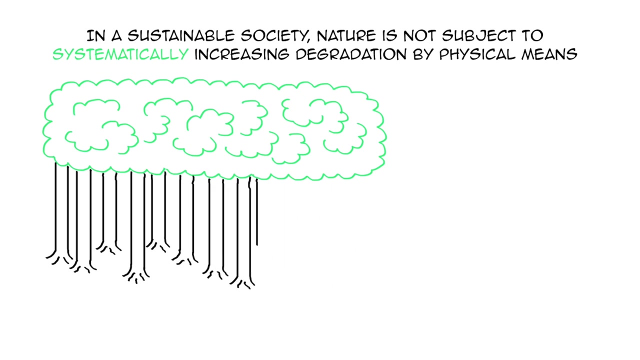 The third principle states: in a sustainable society, nature is not subject to systematically increasing degradation by physical means. This is about how we physically alter nature by way of, for example, logging and fishing. This doesn't mean that we cannot use cut trees or use other resources from nature. We need them to survive. It means that to be truly, 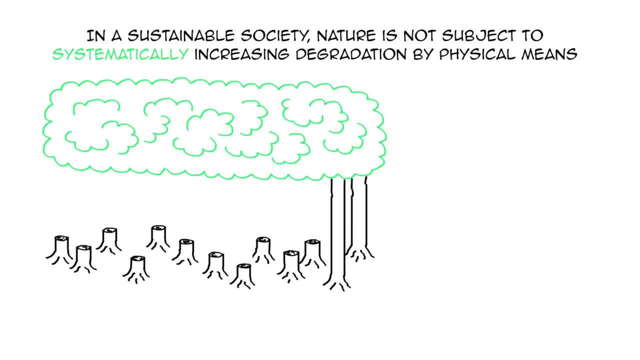 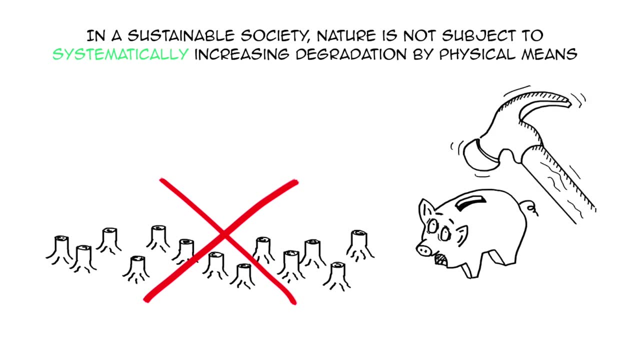 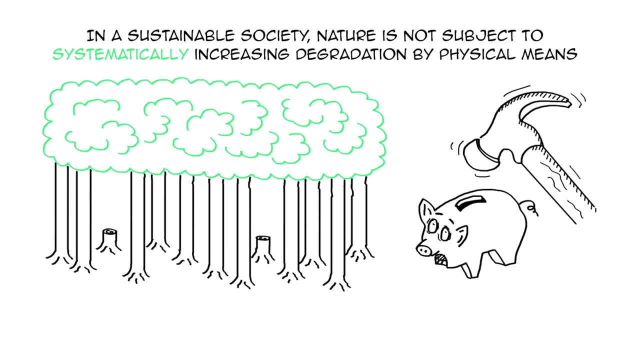 sustainable. we cannot systematically destroy nature at a rate faster than it regenerates. That would be like spending all the capital in your bank account instead of living off your annual revenue. Instead, we have to use our natural resources without exceeding the capacity of the. 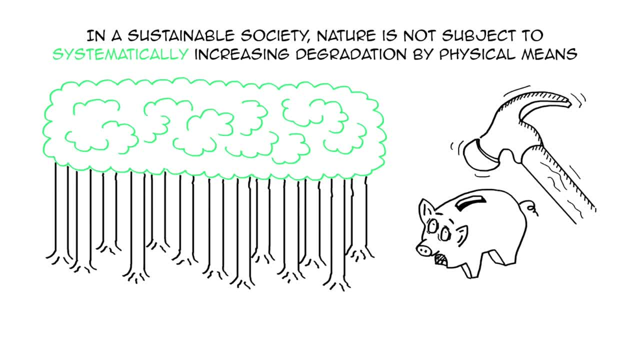 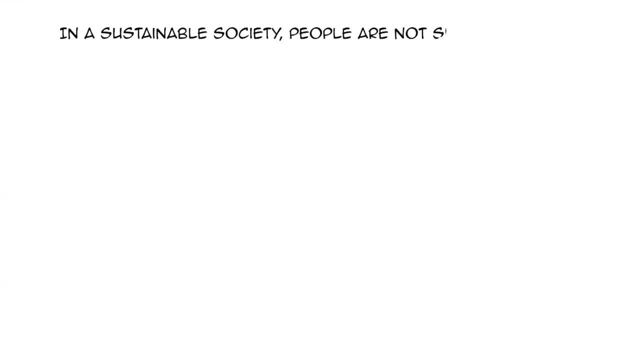 planet to support life on earth. The fourth principle deals with the social aspects of sustainability. It states: in a sustainable society, people are not subject to conditions that systematically undermine their capacity to meet their needs. This doesn't mean that we have to meet everybody's needs all the time. It means that 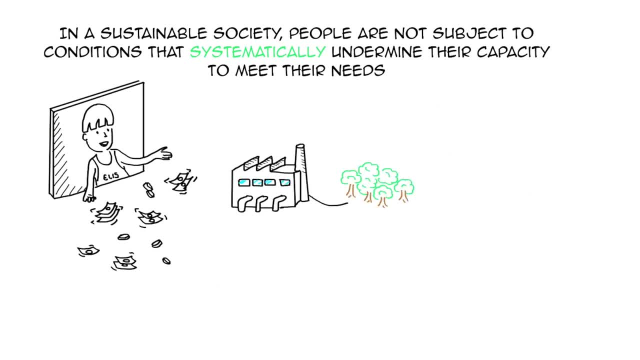 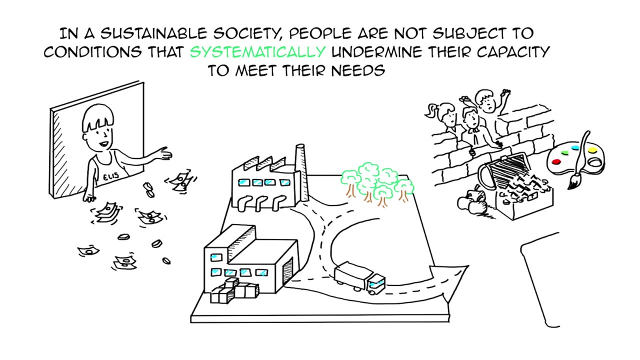 in order to be truly sustainable, we cannot use manufacturing processes, suppliers and business models that create ongoing barriers for people and make it systematically impossible for some of us to meet our needs, such as using exotic mined metals in smartphones, which are now so valuable that civil war is being waged in the Congo to control access to these. 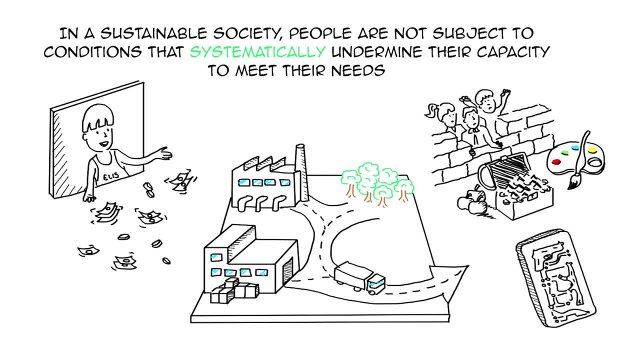 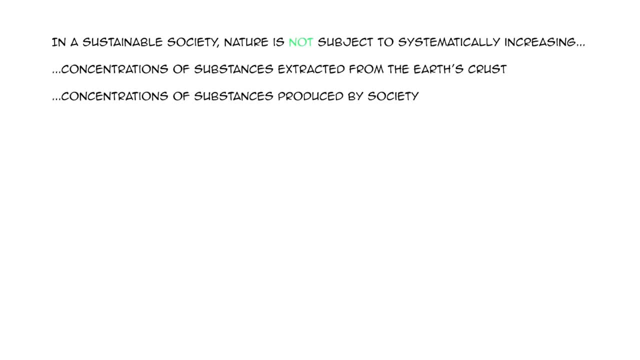 materials. We'll explore the concept of human needs, social systems and social sustainability more deeply in future videos. So here are our four sustainability principles. Together they define checkmate for sustainability, meaning that if our product, our business or our community can truly achieve them, then 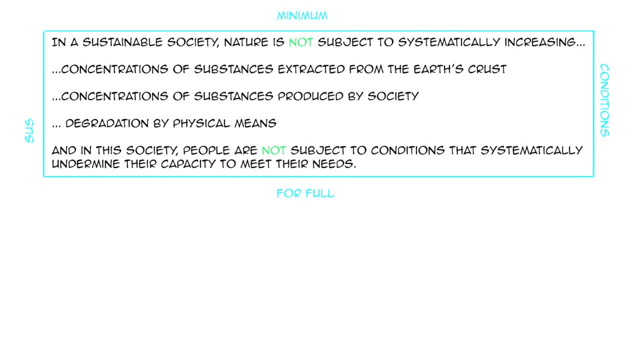 we have achieved minimum conditions for full sustainability. Did you notice that these are the four principles that define the concept of checkmate for sustainability? Did you notice that these are the four principles that define the concept of checkmate for sustainability? The pred 관련 is that they're all phrased in the negative. Nature is not. subject: People. 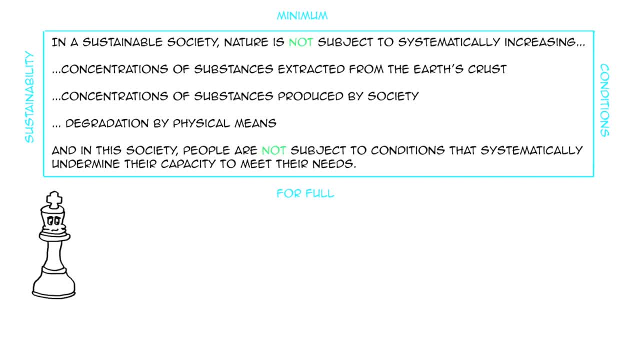 are not subject- Like in chess, the king cannot escape from capture. They're not prescriptive, like. here is the list of the 3,000 things you need to do to be sustainable. These conditions are boundaries, they are the rules of the game. As long we 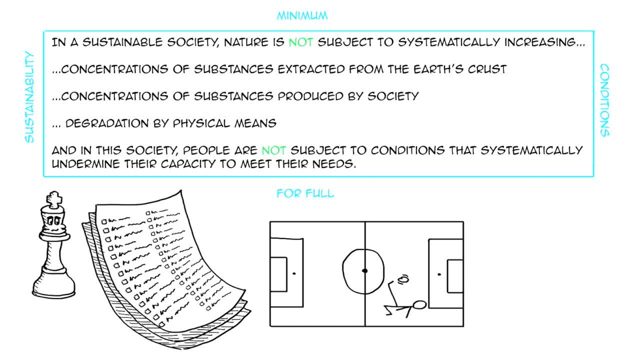 play. within these rules, we can be as creative as we want and invent anything we like. You also noticed that the wording of these conditions is very precise. This is the result of a scientific consensus. They are not designed for communication. I will bring other videos for that. 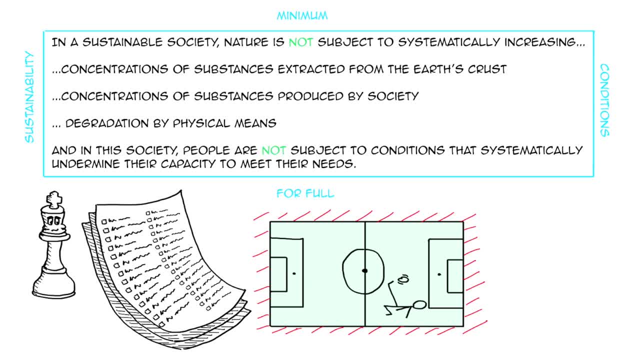 They are here to run in the background, to make sure that we are rigorous when analyzing our decisions and initiatives against a robust framework. They are our North Star, if you like, helping us know where we are and make sure that we are going in the right direction.